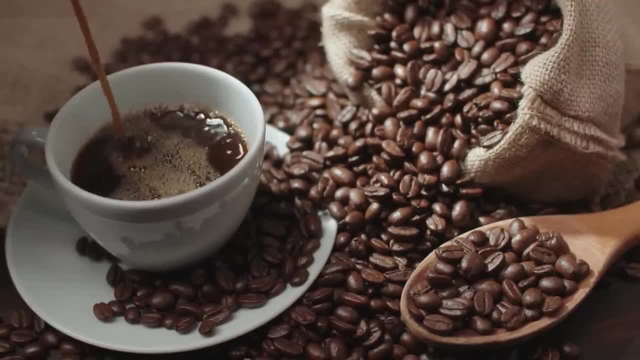 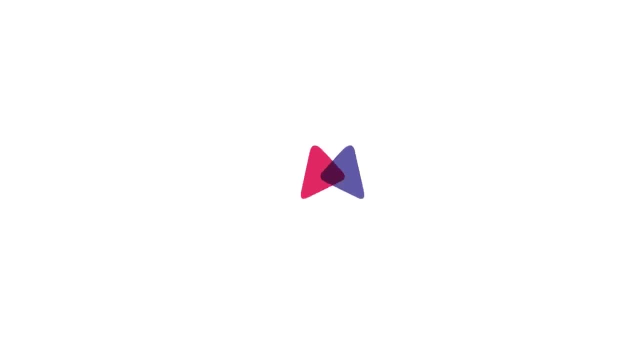 programming language. Also, if you want to learn Java, I have a comprehensive two-hour tutorial for you here on my channel. The link is below this video, So let's jump in and get started. The first sorting algorithm we're going to talk about is BubbleSort. 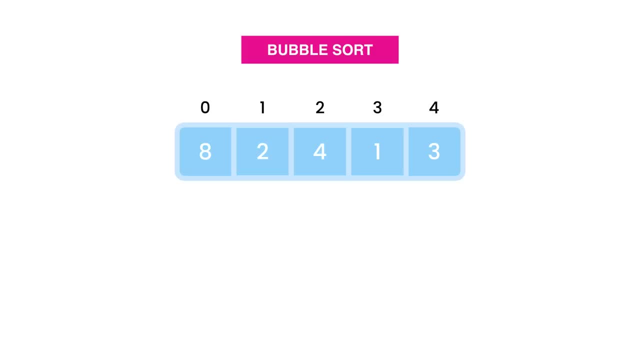 which is the simplest of all sorting algorithms. Let's say we have an area of integers and we want to sort this algorithm. So let's say we have an area of integers and we want to sort this array in increasing order. With BubbleSort algorithm, we scan the 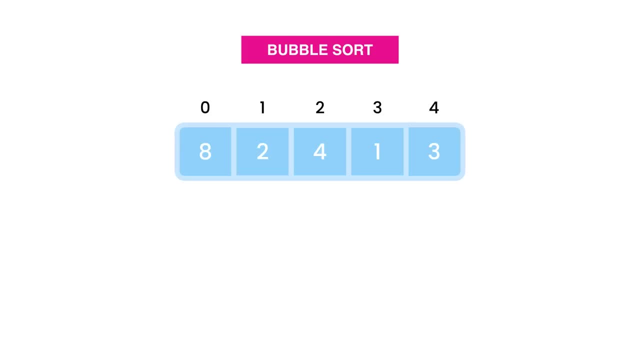 array from left to right, and if items are out of order we swap them. So we start off by comparing the items at index 0 and 1.. If the right item is smaller than the left item, we swap them, because we want to sort this array in ascending order. So here 2. 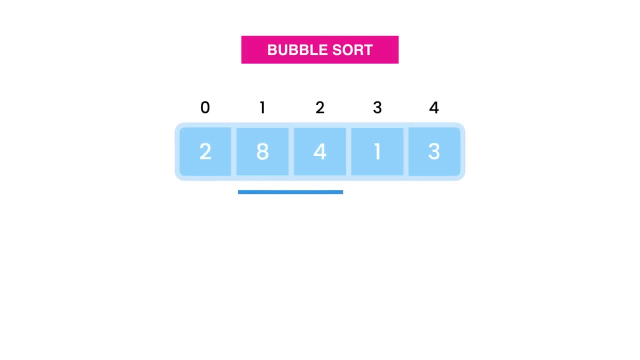 is smaller than 8, and we have to swap them. Now we compare the items at index 1 and 2.. Again, the right item is smaller, so we have to swap these items as well. One more time again, we have to swap these items and. 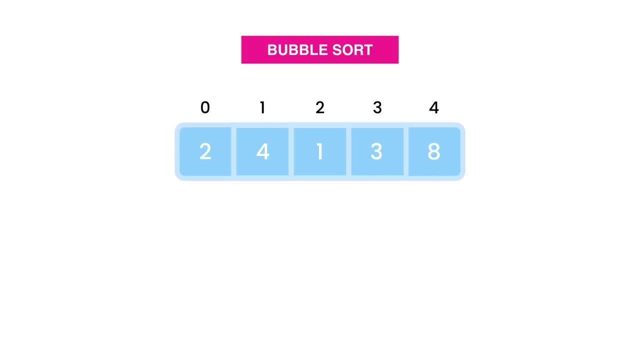 one last time. Okay, this was our first iteration, or first pass. We need multiple passes to fully sort this array. At the end of each pass, the next largest item moves to its correct position. So here 8 is in the correct position. This is why we call this. 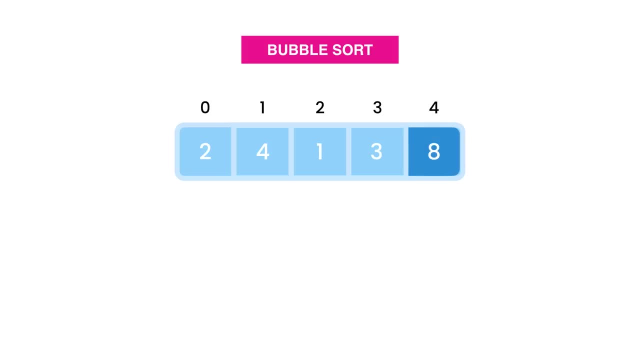 algorithm BubbleSort, because after each pass, the next largest item bubbles up and moves to its correct position. So in the next pass, the next largest item, which is 4, will bubble up. Let me show you Once again. we compare the items. 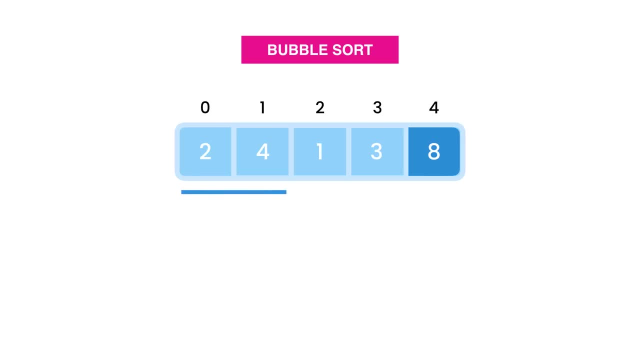 at index 0 and 1.. These items are in the right order because 4 is greater than 2.. So we don't need to swap them. Let's look at the next two items. One is smaller than 4, so we should swap these items. 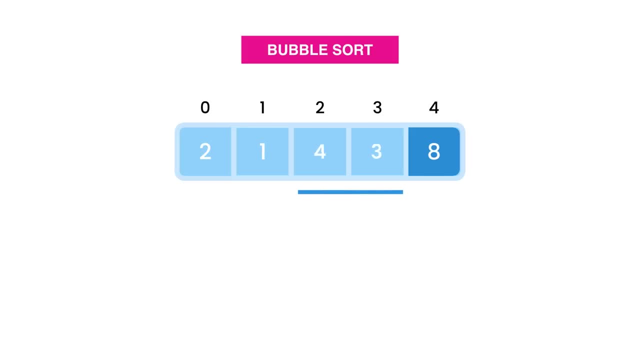 And one more time again: these items are out of order, so we need to swap them. And the last two items. These items are in the right order, so we're done with the second pass. Now 4 is in the right position. 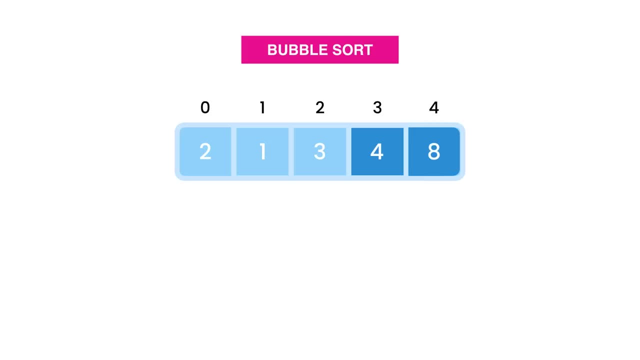 And see, our array is almost sorted. We just need one more pass to swap 2 and 1, and then our array will be fully sorted. So let's do that real quick. Alright, our array is fully sorted. Now let's talk about time complexity, If you're not familiar with this. 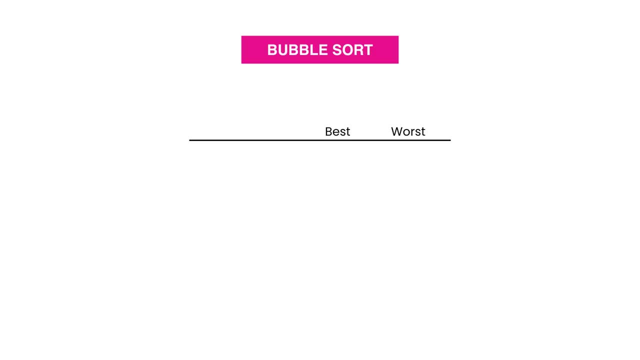 concept, you need to go back to part 1 of this series, where I talk about big O notation. So what's the time complexity here? Well, in the best case scenario, where our array is already sorted, we need a single pass. 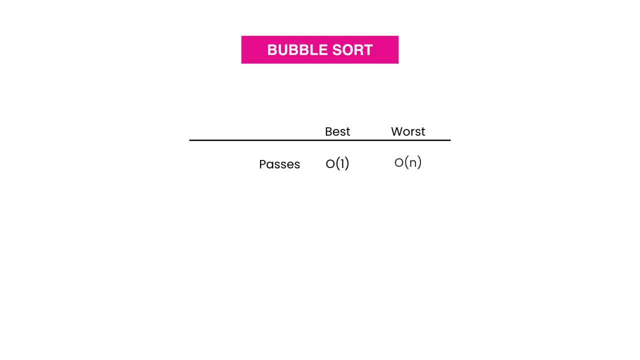 In the worst case scenario, the array is sorted in reverse order. Here we need n passes. Now, in each pass we need n comparisons. Well, more accurately, n-1 comparisons. So if you have 4 items, we need 3 comparisons, right? So bubble sort. 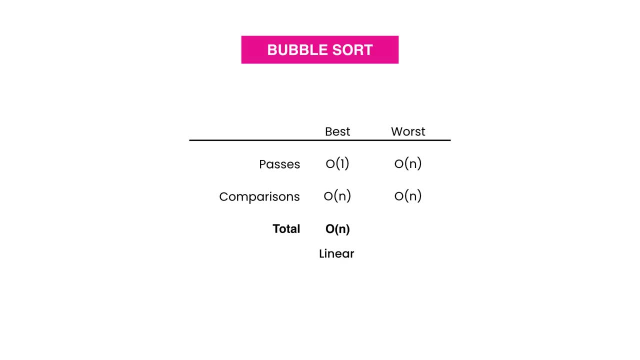 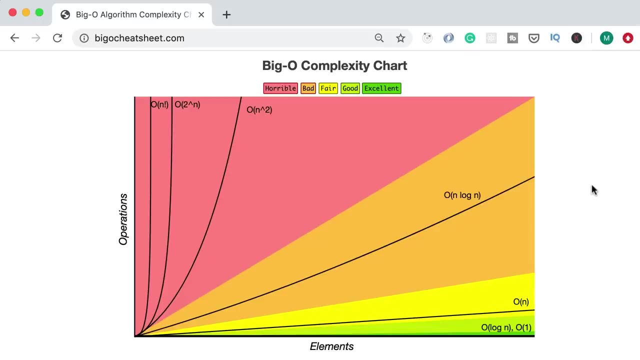 runs in O of n or linear time in the best case scenario, and O of n? squared or quadratic time in the worst case scenario. If you go to bigochitsheetcom, you can see a visual representation of these growth rates. As you can see, O of n- squared is very inefficient. 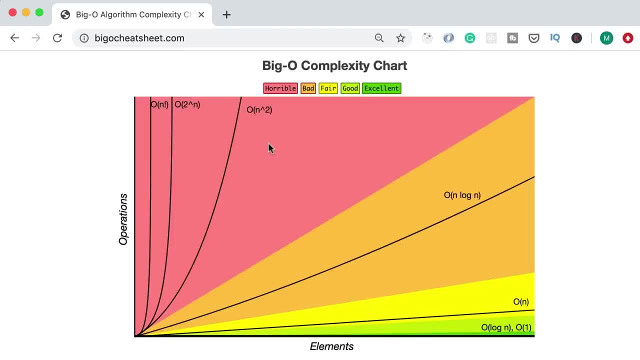 because it's in the red area. So this algorithm gets real slow as the amount of input data grows. Later I will show you better sorting algorithms that run in the orange or yellow areas, But before we get there, let's implement bubble sorting code. So pause the video. 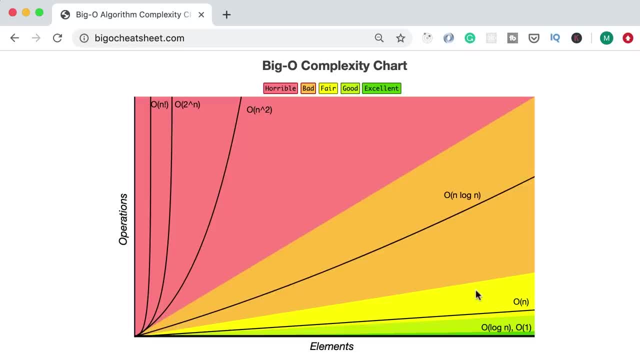 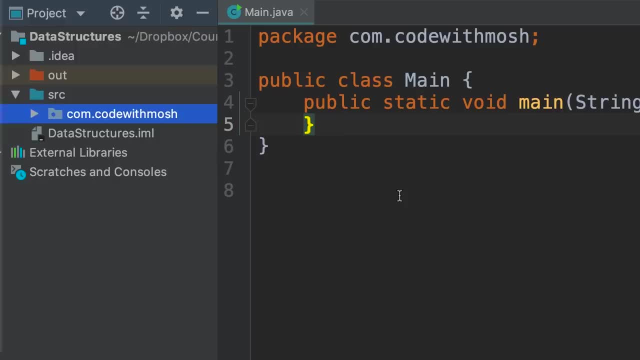 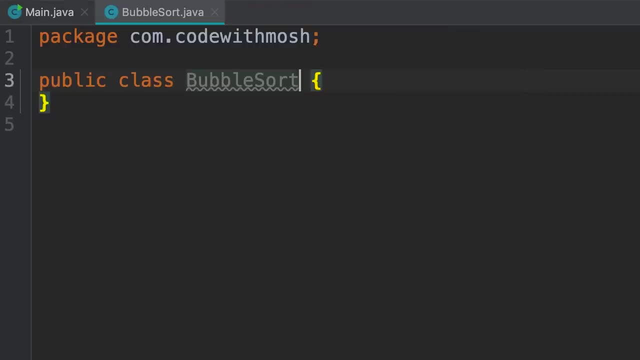 spend 20 minutes and try to implement bubble sort on your own. Then come back and see my implementation. Alright, here in our project let's add a new class. we call it bubble sort. in this class we need one method: public void sort. we give it an. 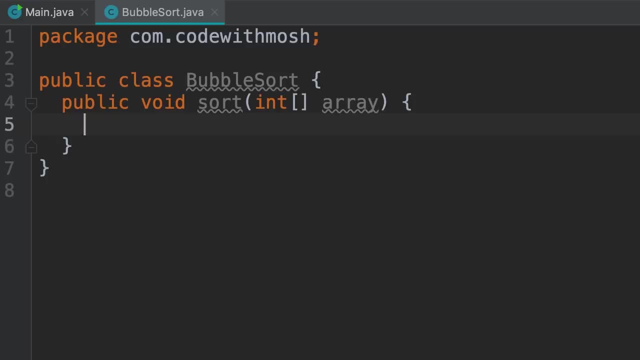 integer array and call it array. Now here we need a loop to iterate over this array multiple times. In each iteration the next largest item will bubble up and move to its correct position. So a typical for loop for i is related to 0,. 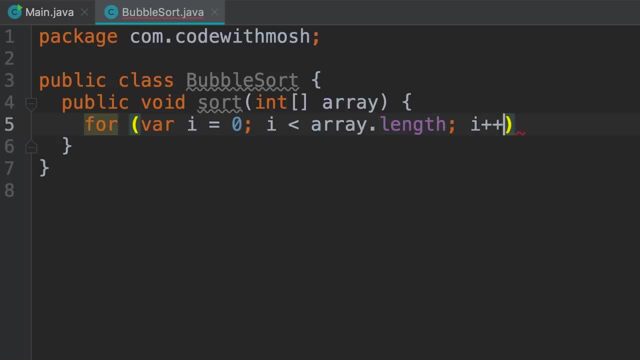 as long as it's less than arraylength incremented after each iteration. Now here we need a second loop, and we use this loop to compare every two items of this array. So let's call this loop variable j. we can set it to 0 and start from the first item, or 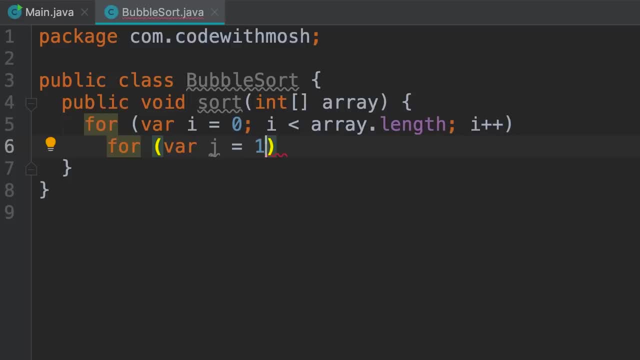 1 and start from the second item. So here we'll compare the second item with the previous item. So we set j to 1 as long as j is less than arraylength we incremented after each iteration. now, in each iteration we're going to compare. 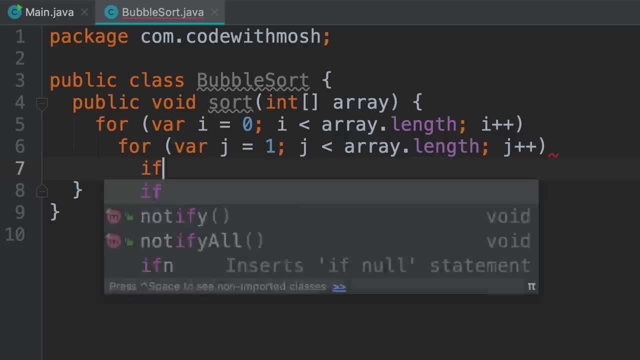 the item at index j with the previous item. So if array of j is smaller than the previous item, that means these two items are out of order. So we need to swap them. How do we do that? Real easy, we've done this before, So we use a. 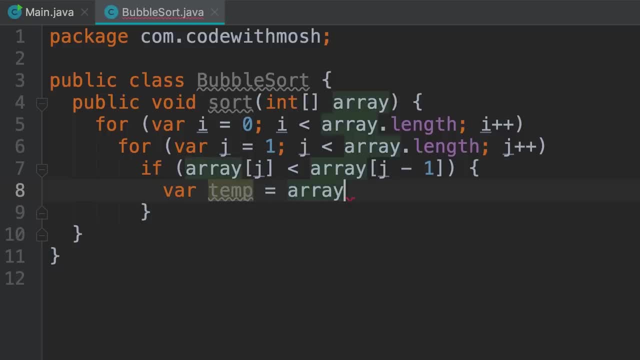 temporary variable and copy array of j into this variable. Then we set array of j to array of j-1, and finally, whatever we have stored in the temp variable, we use that to set array of j-1.. So, array of j-1. 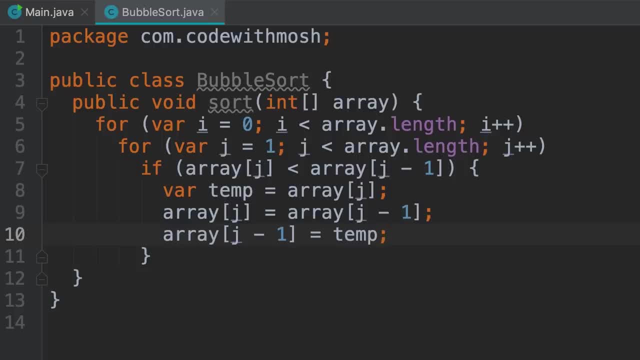 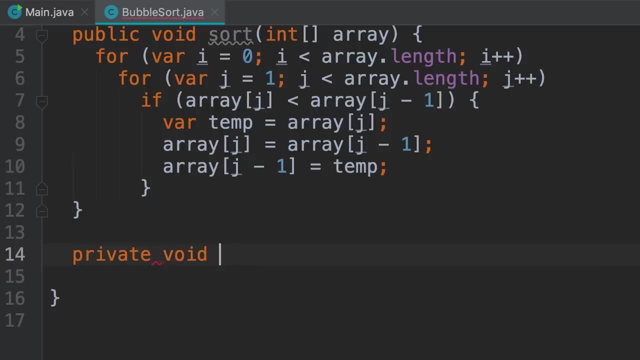 equals temp. That's our bubble sort. Now I prefer to extract these three lines into a separate method called swap. this will make our code cleaner and more readable, So let's declare a private method here. private void swap. we need to pass our integer array. 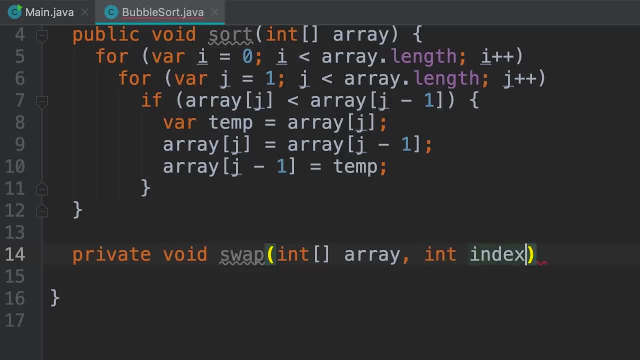 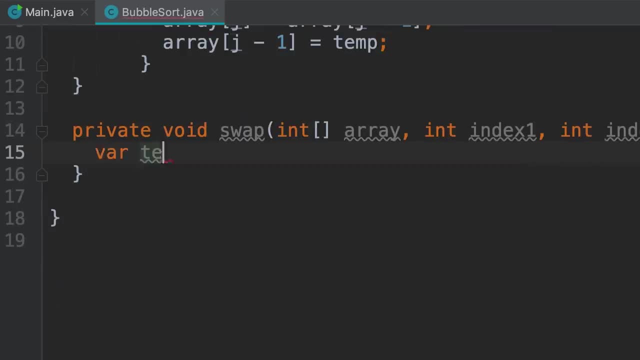 and two indexes, So index 1 and index 2.. Now, once again, we use a temporary variable, so we set temp to array of index 1, then we set array of index 1 to array of index 2, and finally we set 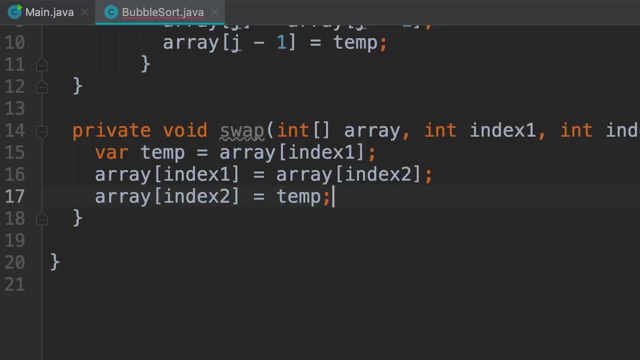 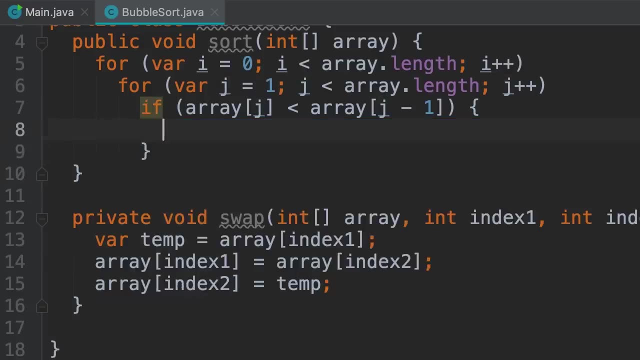 array of index 2 to temp. right Now back to our sort method. instead of these three lines we can call swap, pass our array and two indexes, j and j-1.. Now, because we have a single statement here. 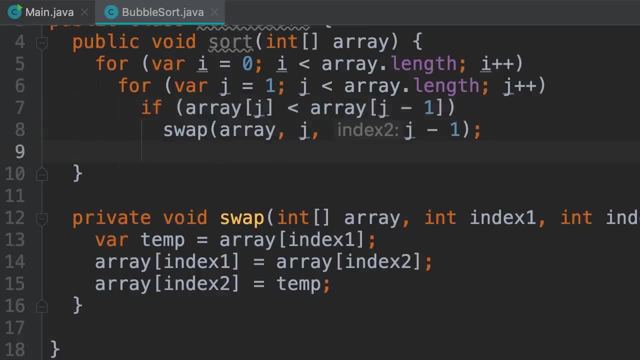 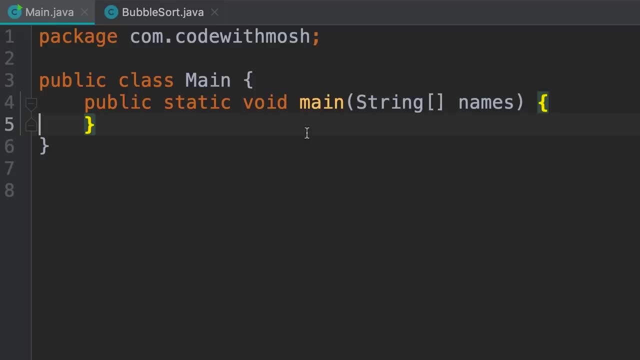 I would prefer to get rid of these ugly, curly braces. that is better. So we're done with this implementation. now let's test it Back to the main class. let's declare an integer array called numbers and set it to 7: 314. 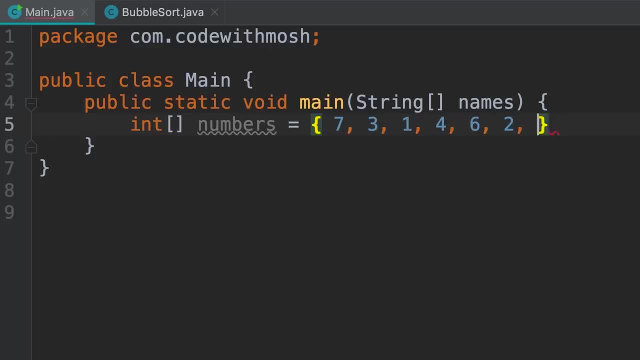 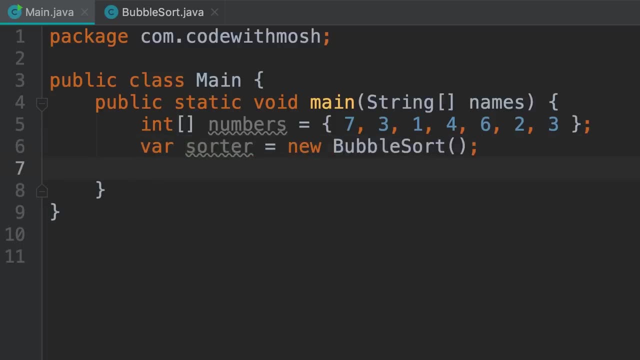 62 and let's add a duplicate like 3.. Now we create a sorter object, we set it to a new bubble, sort, and then we call sortersort, pass the numbers array here And finally we're going to print this on the terminal. So here we use arrays. 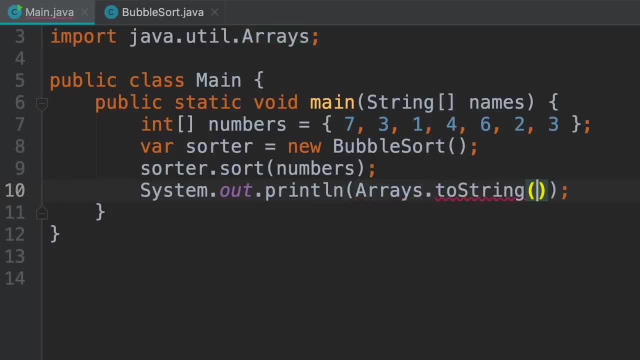 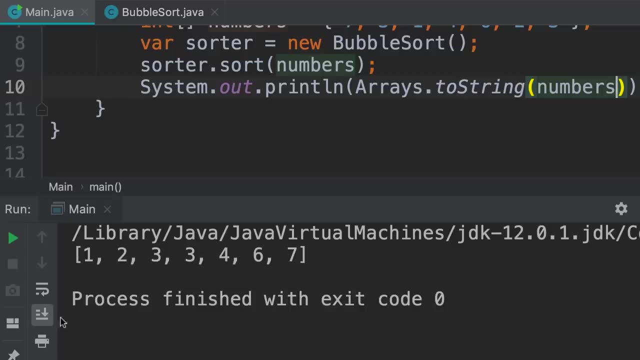 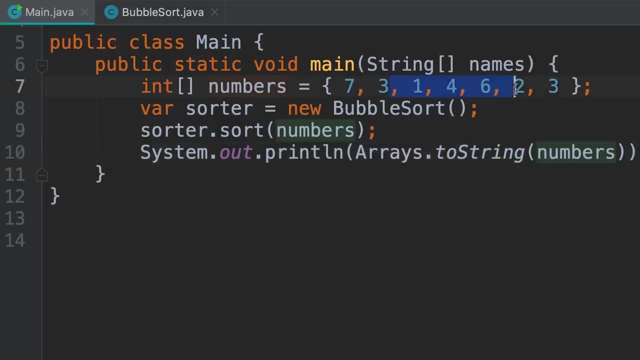 toString to convert this array into a string. so we pass the numbers array and run our program. so, as you can see, our array is sorted. now let's test the edge cases. what if we have, let's say, only two numbers here? our algorithm still works, beautiful. what if you have a single number? 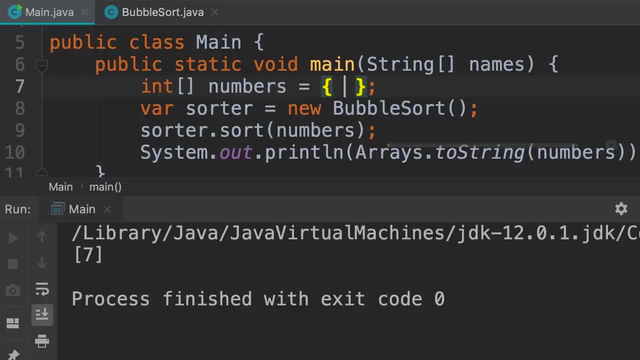 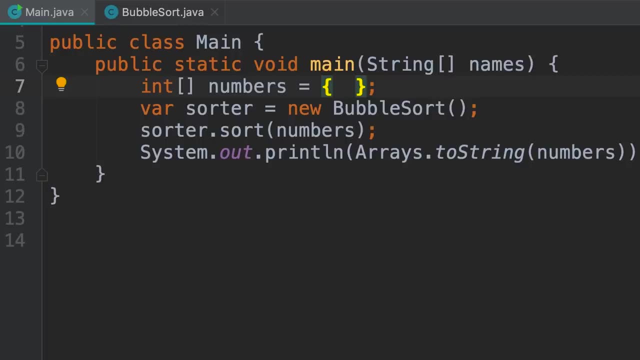 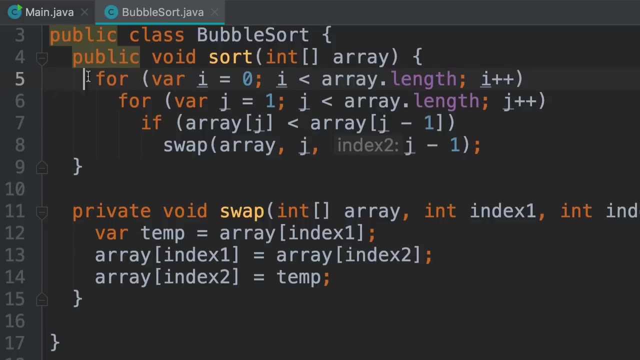 Still working. beautiful. what if you have an empty array? No problem. so we have successfully implemented bubble sort, but there are a couple of places where we can optimize our implementation. let me show you. so back to our bubble sort class. here we are assuming 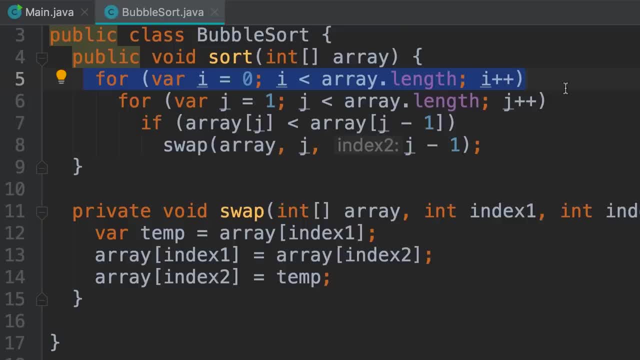 that we need n iterations to sort this array. but what if our array is already sorted or partially sorted? then we're not going to need n iterations, we need fewer iterations. so here I'm going to declare a boolean variable called is sorted. 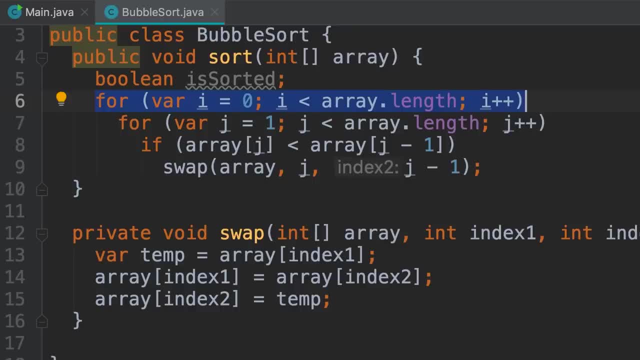 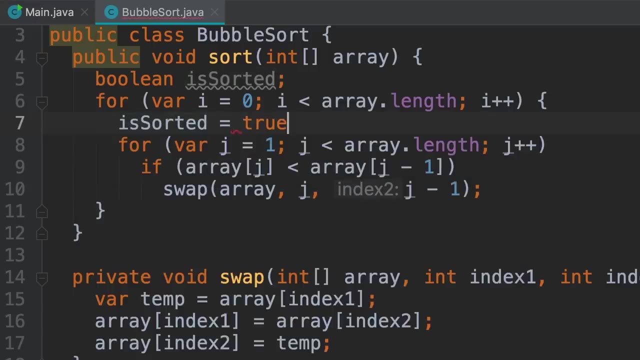 now in every iteration you want to set this to true and assume that the array is sorted. if our assumption is correct, then we'll return immediately. so let's add curly braces here in every iteration first. we set is sorted to true, we assume that the array is sorted now. 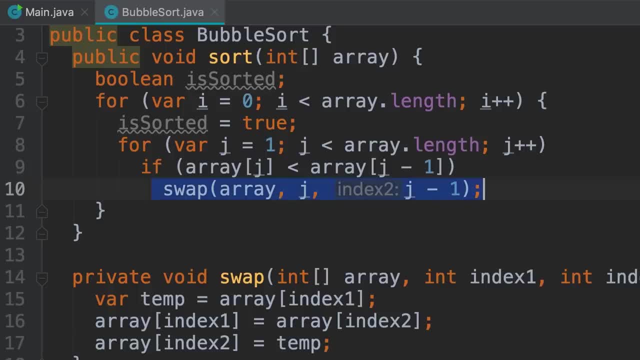 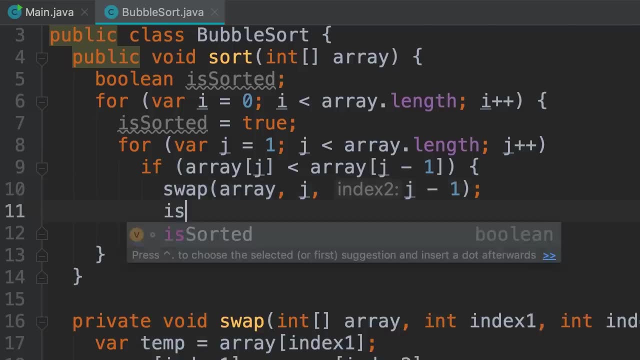 we start comparing items. if we end up swapping two items, that means our assumption was wrong. so right after swapping we need to set is sorted to false. however, if we don't do any swaps, that means our array is fully sorted. so 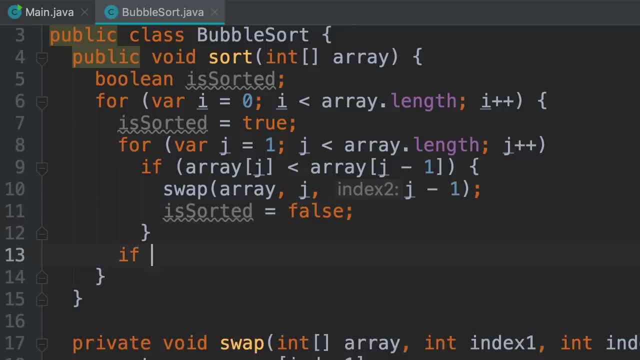 after this for loop, we can write an if statement. if the array is sorted, we can return immediately. there's no need to iterate over this array one more time. that is one optimization. we also have another optimization. look at this inner loop. here we are going through the entire array, comparing every 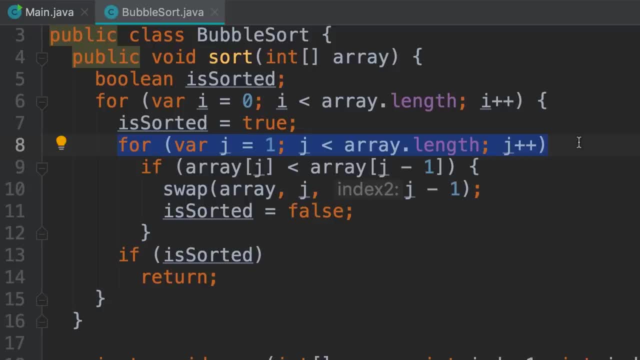 two items. but, as you learned in every iteration, in every pass, the next largest item bubbles up and moves to its correct position. so we don't really need to compare all of the items in this array, we only need to compare all the items. 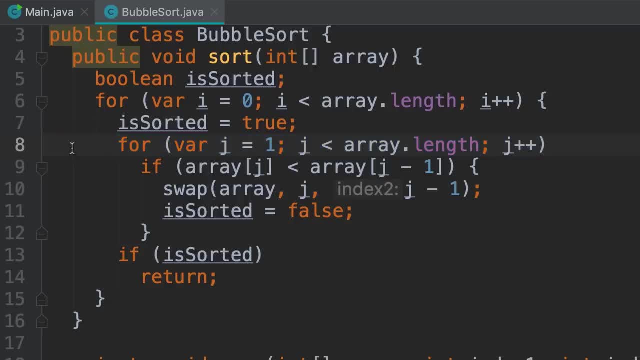 that are not in the correct position. So in our first pass no items are in the correct position. that means we should iterate over all the items in this array. in the second iteration one of the items is in the correct position so we need to look at all the items except the last.